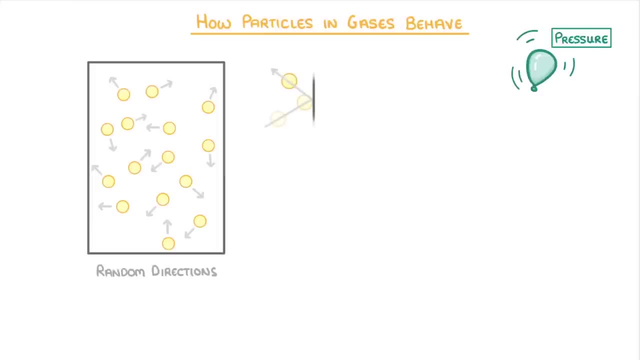 on in a different direction. Even though they're tiny, the particles still exert a force whenever they collide with the walls of the container, And this means that they create pressure, as pressure is just the force being exerted per unit of area or the force divided by. 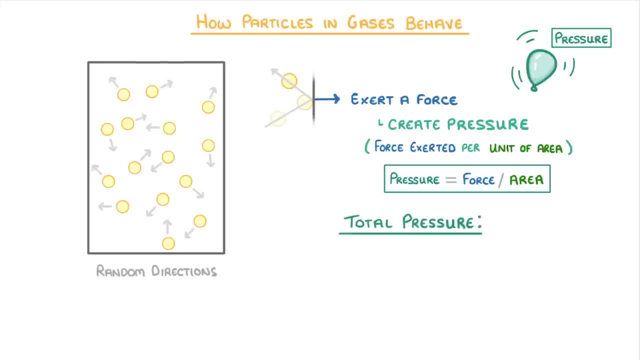 the area. The total pressure, though, is going to depend mainly on two things: how many of these collisions there are and how much energy each collision involves, And we can use these principles to understand how the temperature, the concentration and the volume each affect the pressure. 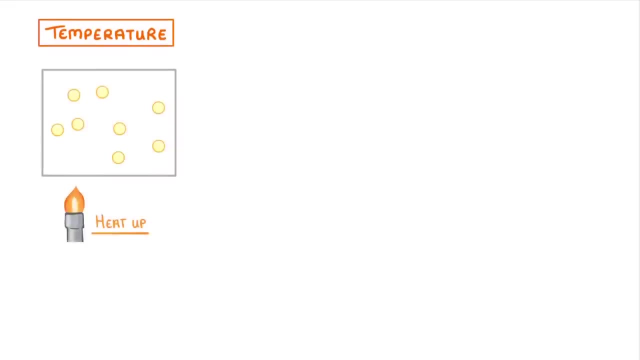 Let's start with temperature. If we were to heat up our gas, we would be transferring energy to the particles, kinetic energy stores, So all of our particles would start to move around faster. And because they are all moving around faster, there would be more collisions with the walls. 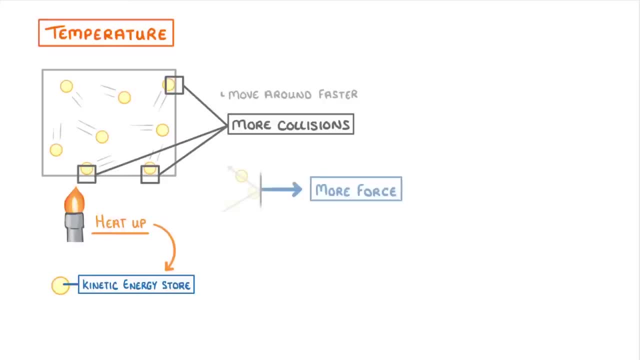 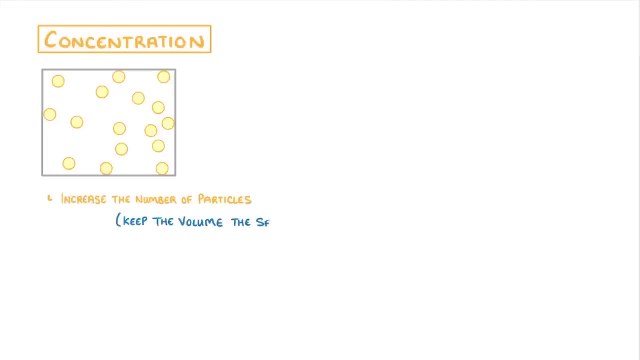 of the container and each individual collision would involve more force, Because these are the two important factors that determine pressure. we can be sure that pressure increases with temperature. Next up is the concentration. If we increase the number of particles in our container but we keep the volume, the 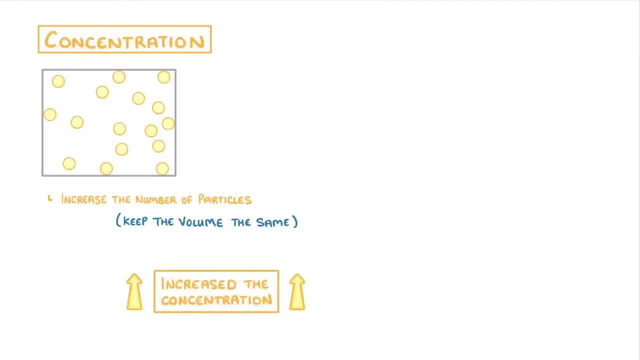 same, then we've effectively increased the concentration, and so there will now be more particles to collide with the walls. This means that there will be more collisions, Which again means that there will be more collisions. Finally, we have volume. If we made our container smaller but kept the number of particles the same, then there 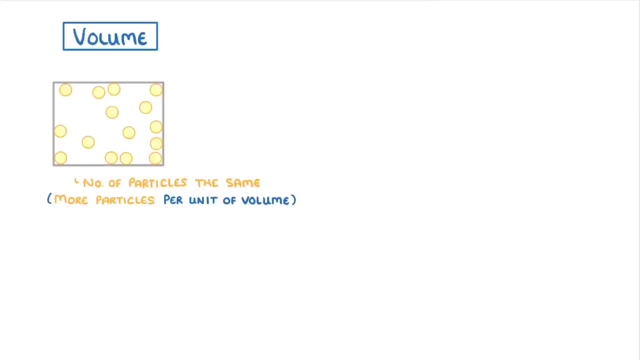 would effectively be more particles per unit of volume, Which is actually the same thing as saying there's a higher concentration of particles. As the particles no longer have as far to travel between each collision, there now could be more collisions, meaning a higher pressure. 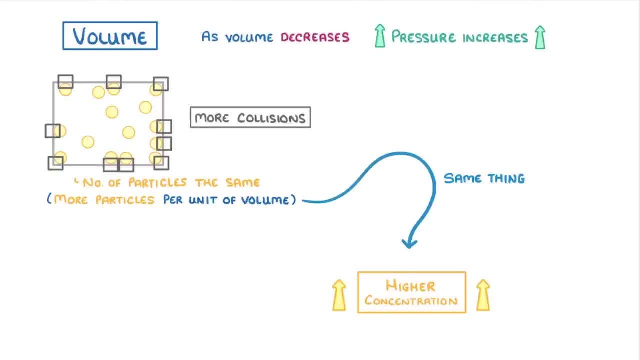 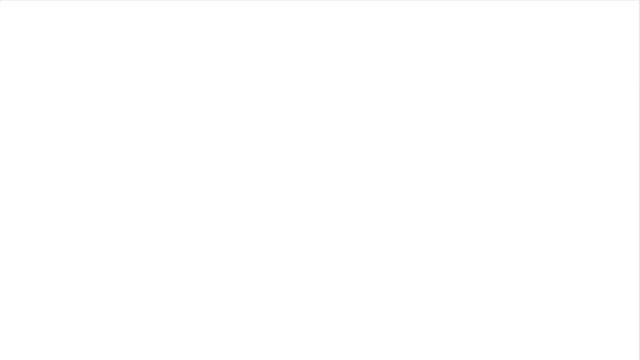 So, as volume decreases, pressure increases. The last thing I want to mention is that we've so far been considering our containers as a fixed shape. Sometimes, though, like in the case of a balloon, the container is flexible, and so it can expand.